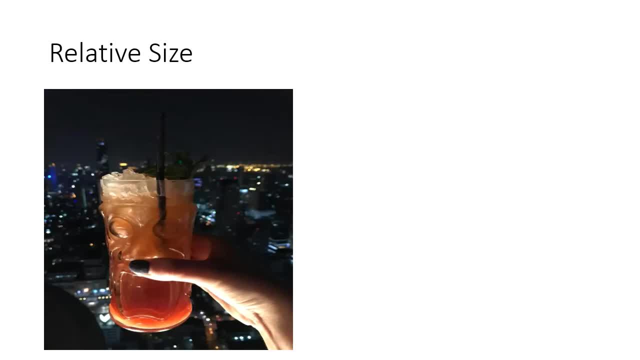 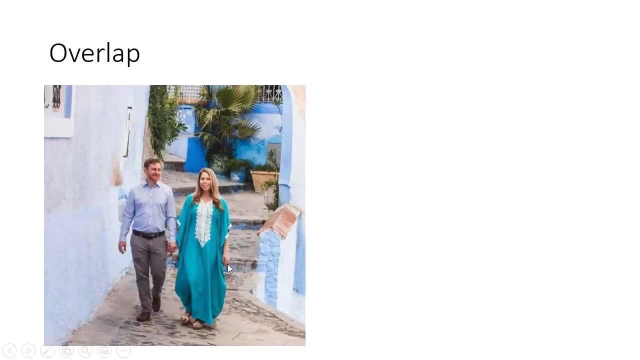 So things that are further away appear smaller. That is an example of relative size, So I'm going to jump to the next one. This is overlap, So see how the stairs going up are. my wife's face is being shown over the stairs and my face is being shown instead of the stairs. So when we're overlapping, but you can see me instead of the stairs And that's a sign that I'm closer to the stairs. 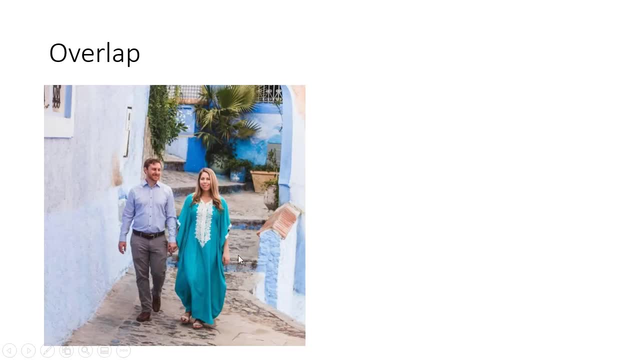 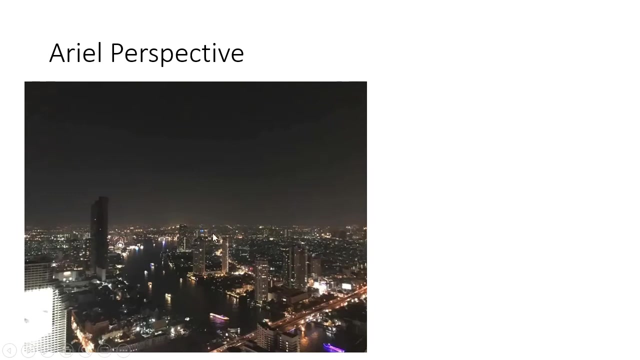 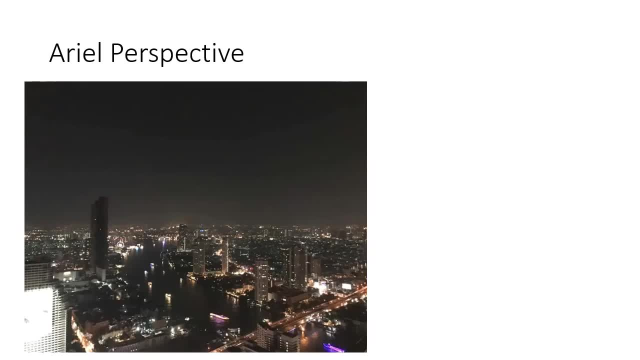 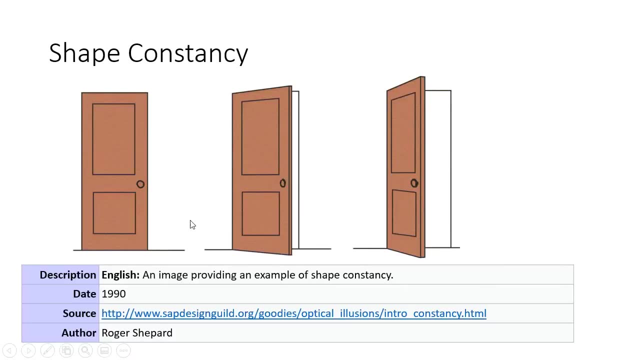 things get blurrier as you look further into the distance. and then I'm gonna go ahead and jump to the next slide. so this is shape constancy, and so it's the idea that, even though the actual shape of something changes based on how an object is positioned, we still generally perceive it as the same shape. so with a 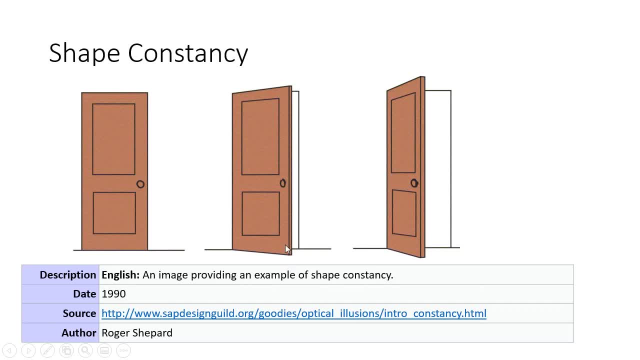 door, we still perceive it as a rectangle, even though here, when the door is slightly open like this, it actually is a trapezoid. so see, and then here it's even more like a trapezoid, even though, so even though, it changes positions and the 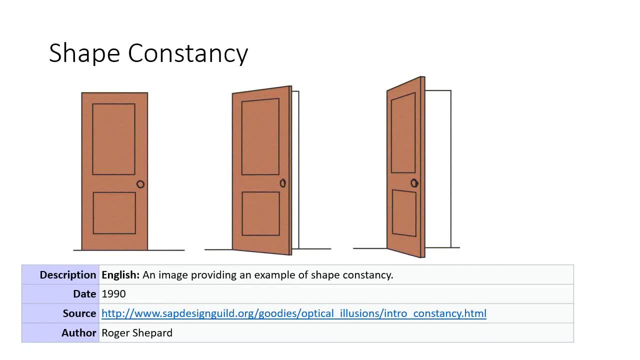 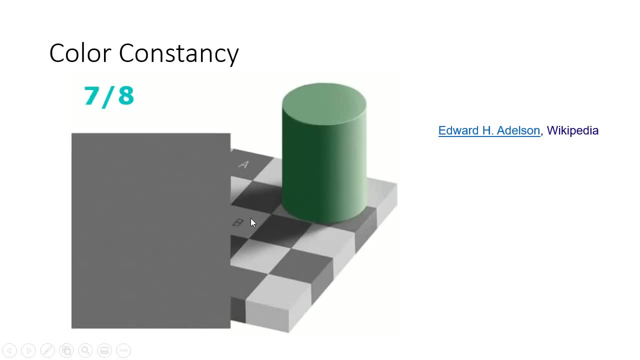 shape looks different, we still perceive it as a rectangle. this is color constancy. so right here, this is kind of a famous one. so you can see that that this, this shape or this color here, even though it's darker, appears whoops. this color here. it appears the same as this color here, even though they're different. 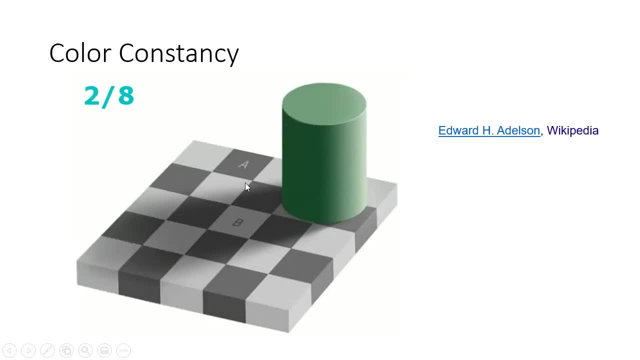 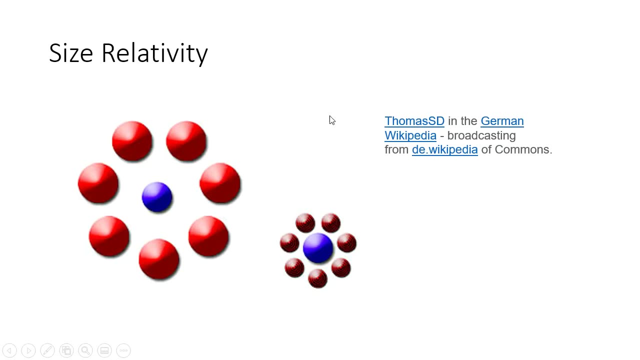 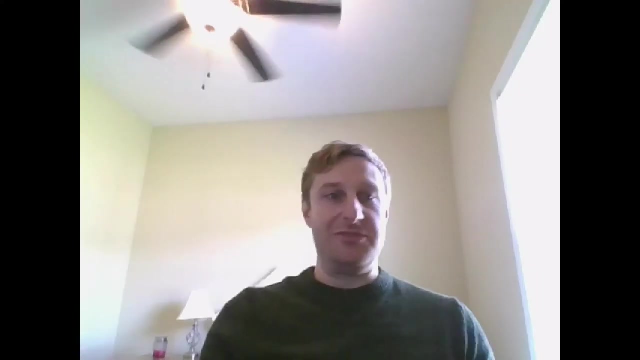 colors. because of the shadow, they appear the same and that's called color constancy. so there I'm going to talk about some illusions real quick. so size relativity is one illusion, so- and this is with color too. so if you based on how certain things are surrounded, that can. 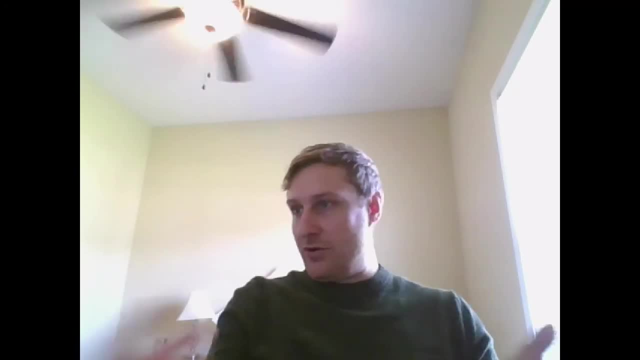 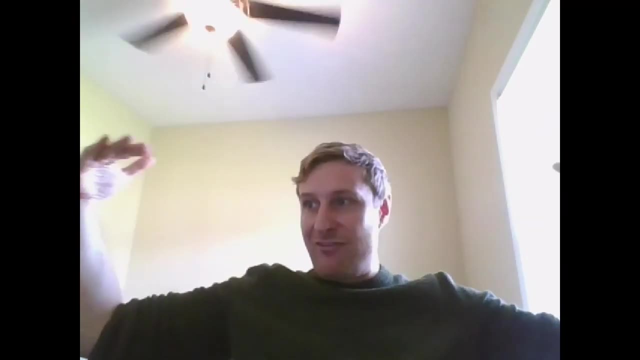 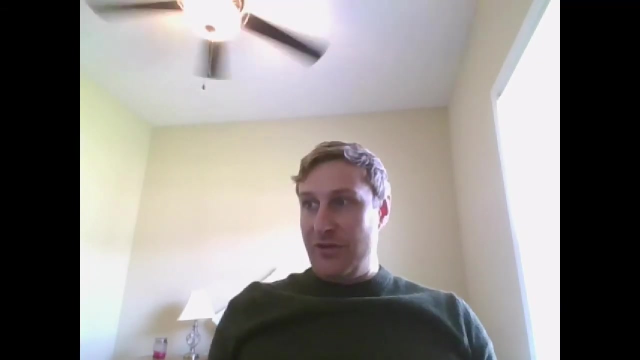 affect your perception of you know, the color, size, whatever, right. so if you're surrounded by a bunch of really tall people and you're an average height, you're gonna look short, you know, compared to to. you know, even though you're not really short, you're just around a bunch of tall people but you're. 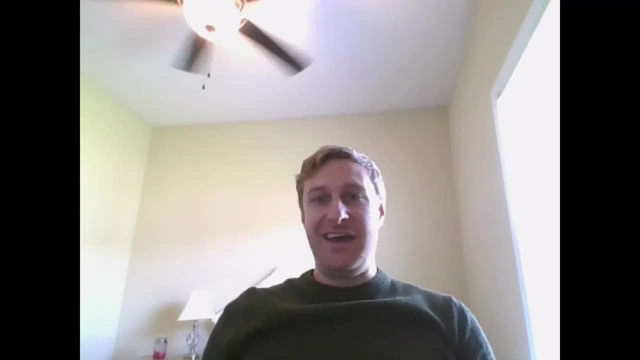 just gonna look short, you know. so, for example, like you may see a bunch of basketball player who's a guard and you're like: oh, he's really tall and really short. And then you see him in person. He's actually at 6'6" And he just appears short because on TV he's standing. 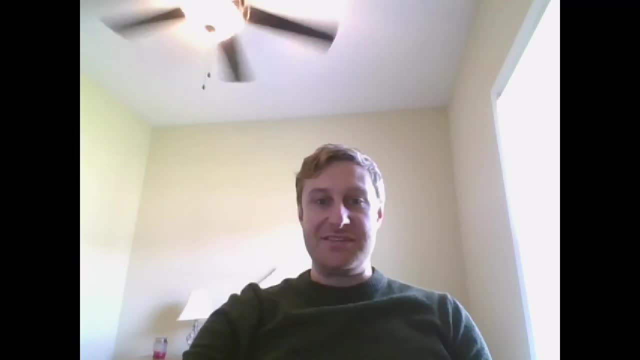 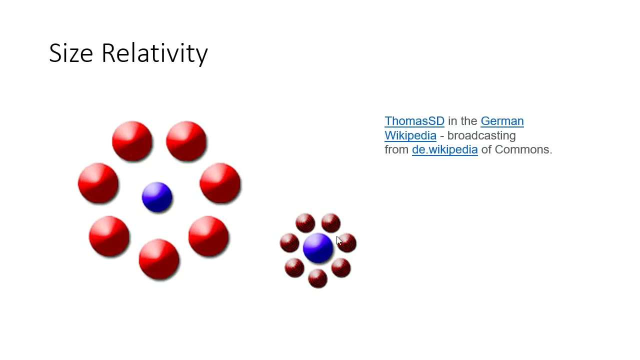 next to all these big, tall basketball players. So this is a good example of that. So you can see, here there's these big circles around this blue dot, And here there's these little circles. This one looks bigger than this one, but really they're the same size, right, And so it's just. 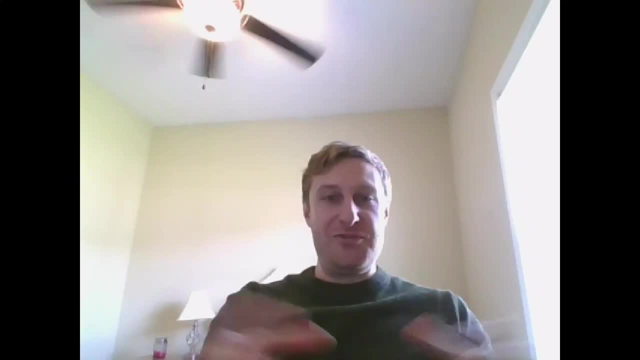 who you surround yourself with. So another example is: maybe if you go out, if you have a bunch of friends who are really ugly and you're okay, average looking, you're going to look more attractive than if maybe you're with a bunch of friends that are really attractive. 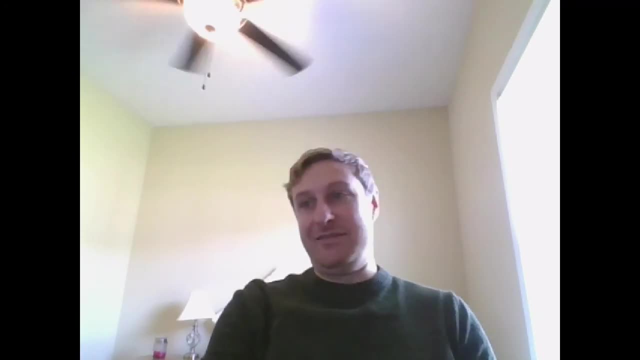 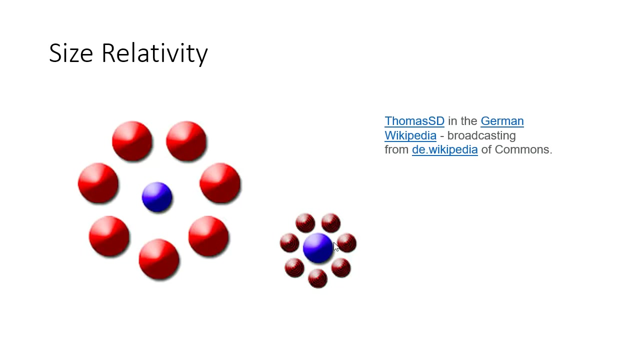 You may, and you're average looking. you may look a lot worse because you're around all these people that are really attractive. So we tend to do that, We tend to compare people to things that are around us, And that's how we make judgments. We can't really 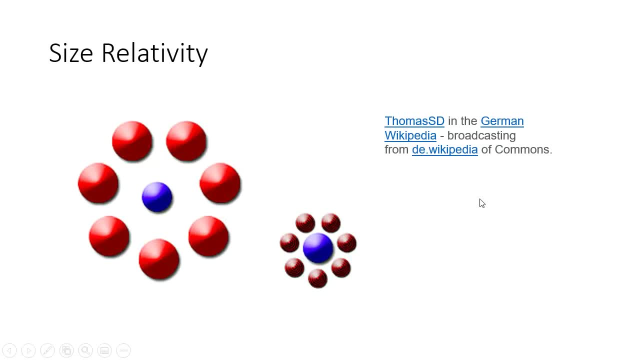 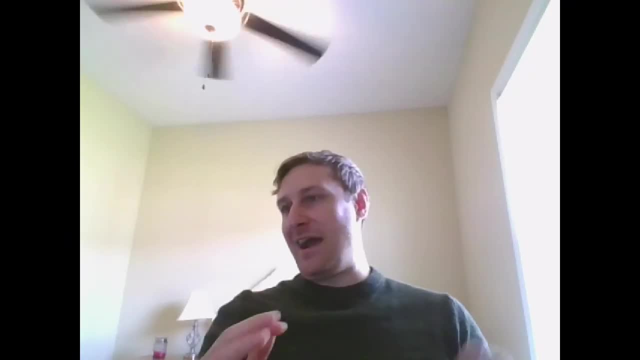 make a judgment without other things to compare it to right. So it's funny, because I'm 5'7" and I was sitting at the back of a pool. We were playing volleyball and I was with. I had all these shorter people in my group and all the taller. 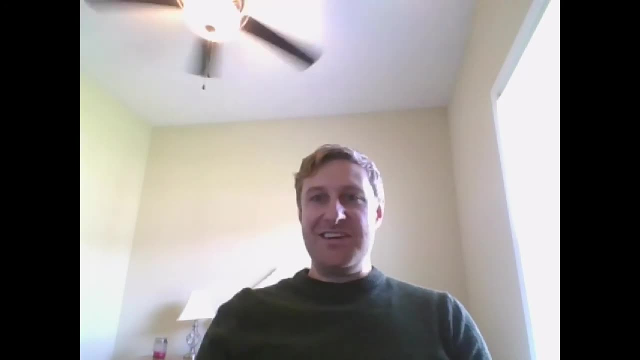 people were on the other side And I said something like: yeah, I'm actually really I feel tall back here. And my friend who's like 6'4", 6'5" said: in the land of the blind,